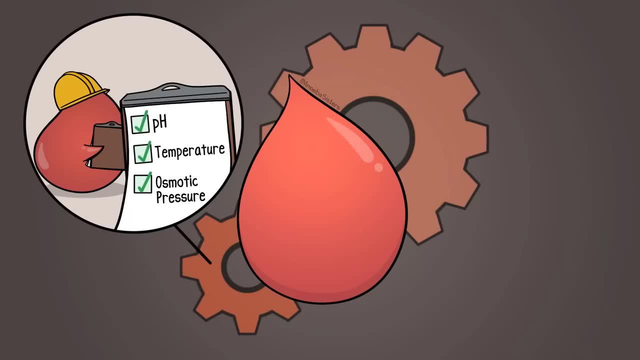 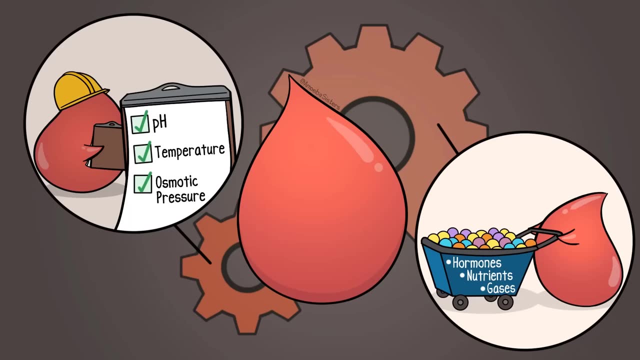 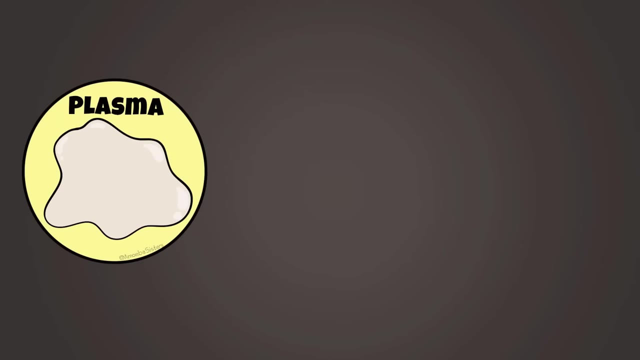 Human blood has a lot of functions. It maintains a certain pH, temperature, osmotic pressure. All of this is very important for homeostasis. It transports things like hormones, nutrients and gases, And it's made up of different components. One component includes plasma. 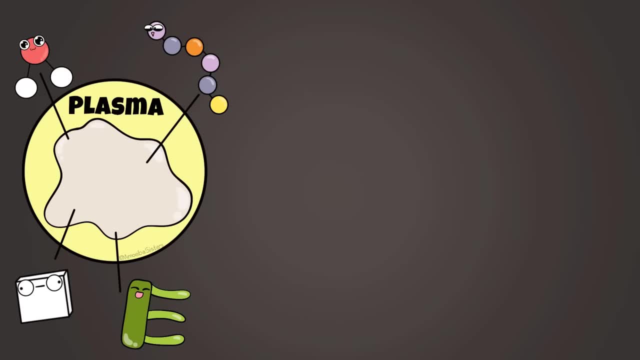 water, proteins, salts, lipids. You'll find them in this liquid portion of blood known as plasma. Another component includes cellular components. This means red blood cells, which do the transporting of gases, white blood cells which can fight infections, and platelets. 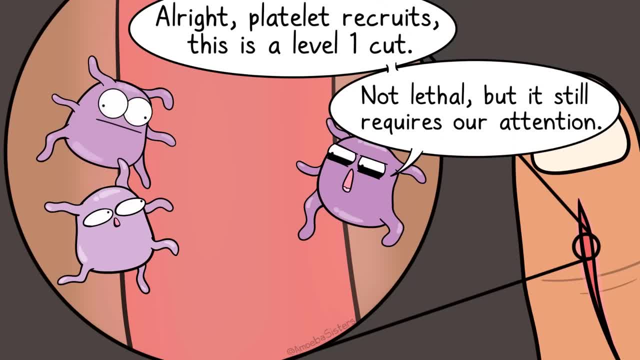 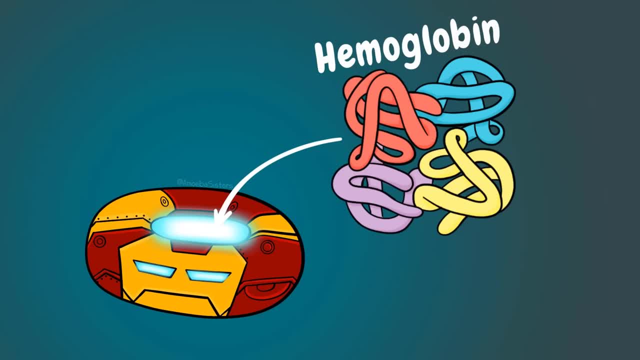 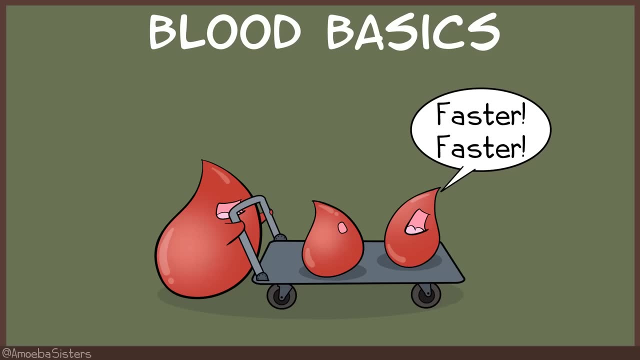 which are actually cellular fragments, and they're involved with helping your blood clot- Very important when there is damage to the body. Red blood cells have an iron-containing protein called hemoglobin and that is where the red coloring of blood comes from. So when we're talking about blood and we're just intro-ing, 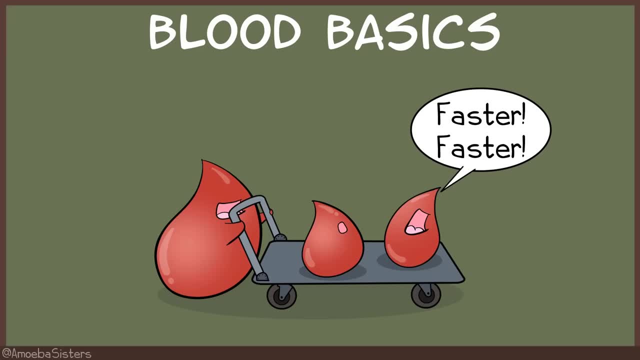 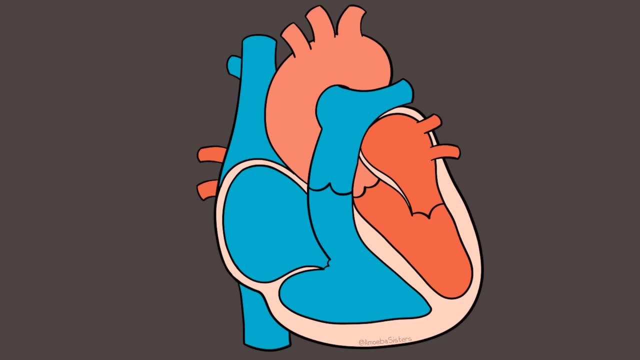 the circulatory system. we're going to focus on how this blood moves around in the human body. Human heart anatomy observes the heart divided into two distinct and separated partitions: A deoxygenated or low oxygen partition and an oxygenated partition. There are some human 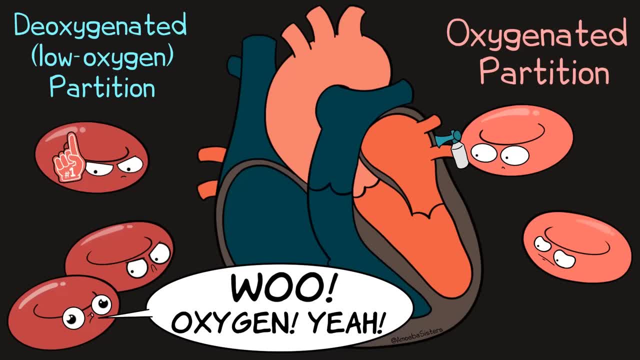 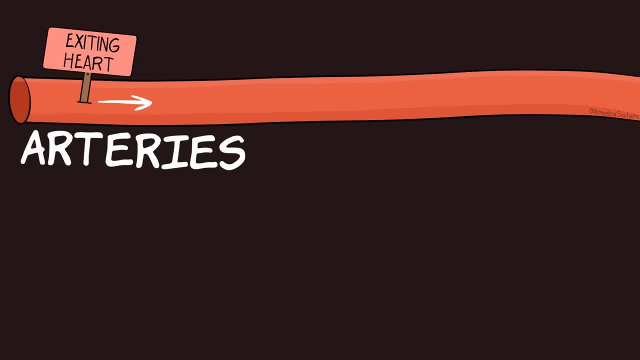 congenital heart conditions that can result in this oxygenated and deoxygenated blood mixing. however, More on that at the end of this video. Arteries carry blood away from the heart. Think A4 away. Arteries are typically oxygen-rich. 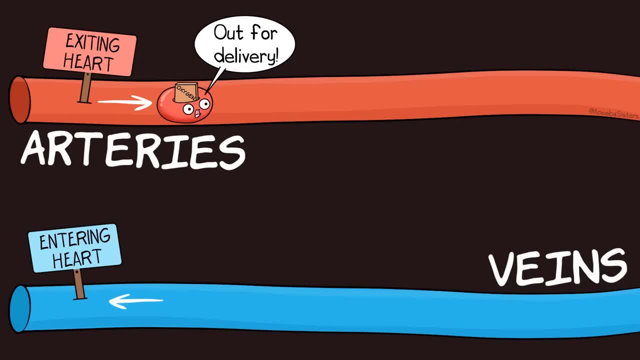 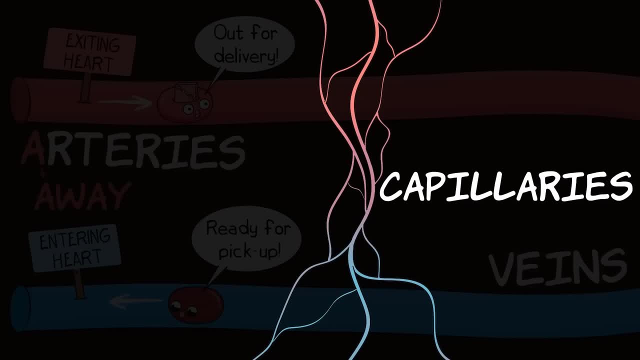 but there are exceptions. Veins generally carry blood to the heart. Veins typically are oxygen-poor, but there are exceptions. Capillaries are small blood vessels and it is at the capillary level where oxygen is delivered to organs and tissues and where carbon dioxide will be picked up to travel. 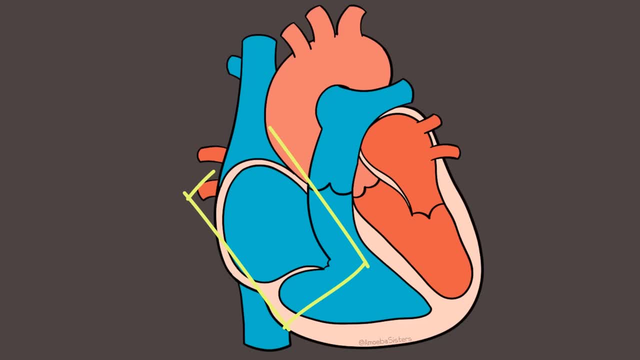 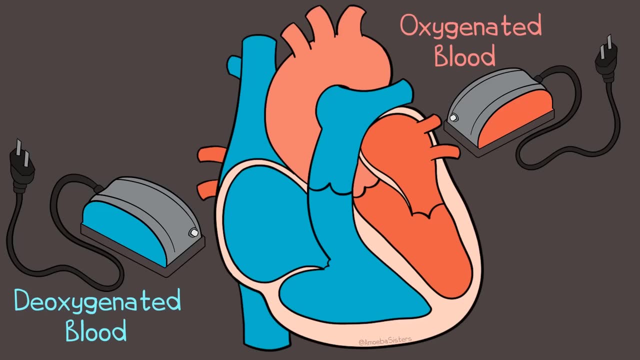 back to the lungs. So, looking at this heart, The right side- and that's the person's right, so for you it will look opposite- pumps deoxygenated blood and the left side pumps oxygenated blood. We can also see four chambers. 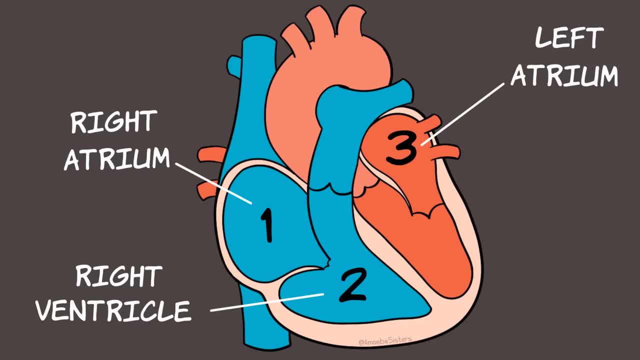 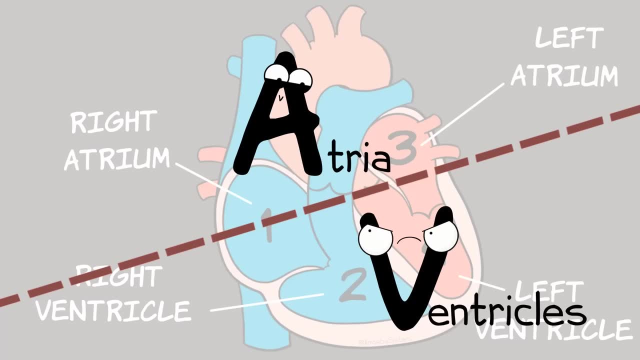 the right atrium and right ventricle and the left atrium and the left ventricle. I like to remember that A comes before V in the alphabet, so that helps me remember that A's for atria are at the top of the heart, V for ventricles are at the bottom of the heart. Atria also. 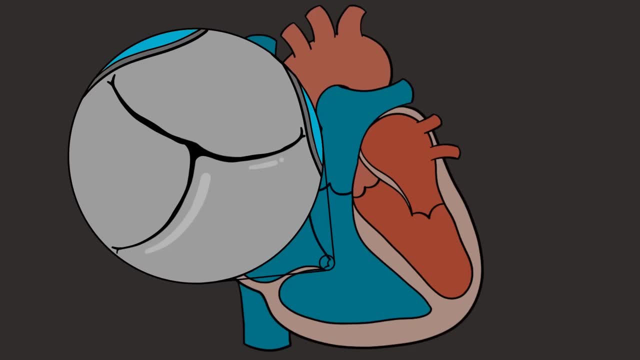 have thinner walls than the thicker walled ventricles. The heart also contains valves, which we'll see when we get to tracing the pathway of blood. The valves are one-way structures that help to separate the chambers And also prevent backflow of blood. 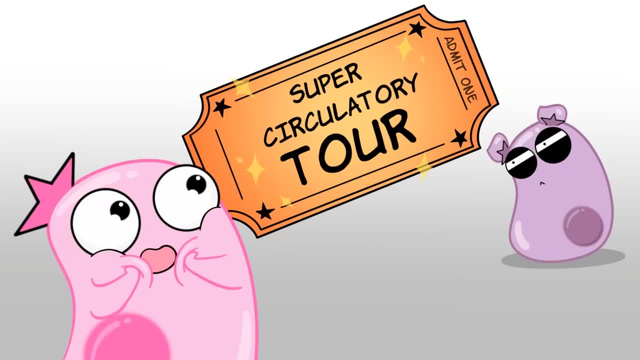 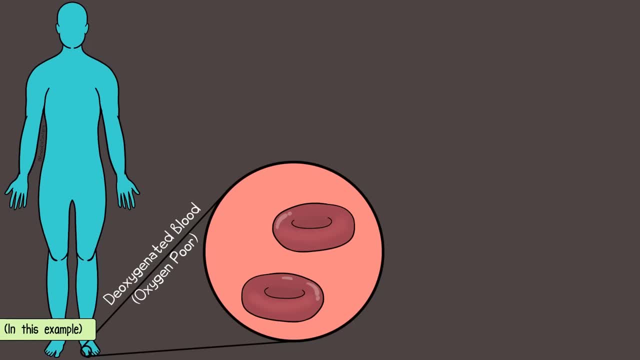 Ready to take the adventure of a lifetime, An adventure tracing the pathway of blood through the heart. We're going to start with blood that is in a human toe. This blood is deoxygenated. It needs to get to the heart so that it can be pumped to the lungs to pick. 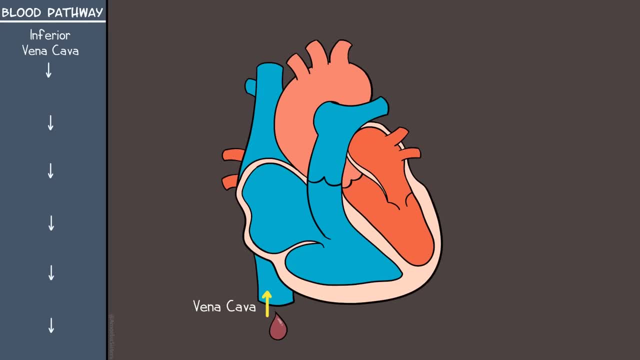 up oxygen and then be spread throughout the body. It's a work that takes a lot of time. Its a bit complicated, but it is a work that you can easily do. Funny, it is such a big work going to get there through the vena cava- inferior vena cava to be specific- as the 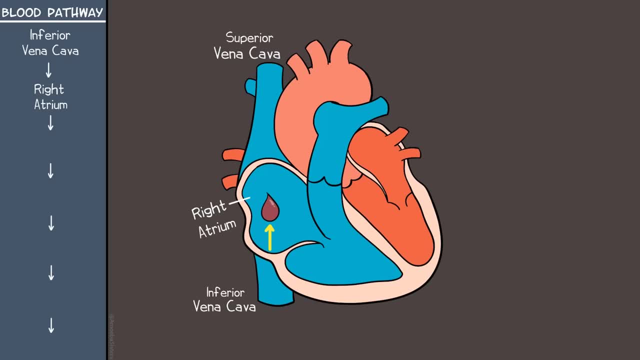 superior vena cava is above the heart. the blood enters the right atrium. the right atrium contracts pushing the blood through the tricuspid valve into the right ventricle. the right ventricle contracts pumping the blood through the pulmonary valve to the pulmonary artery. by the way, when you see the word 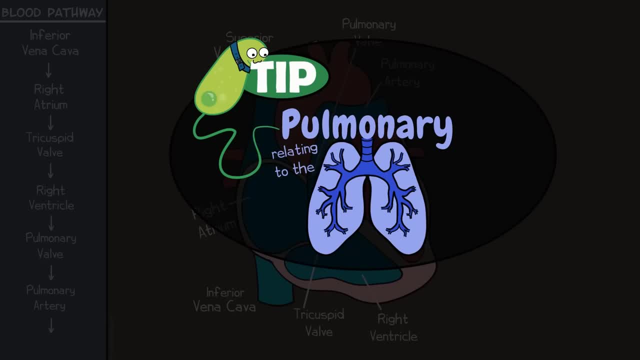 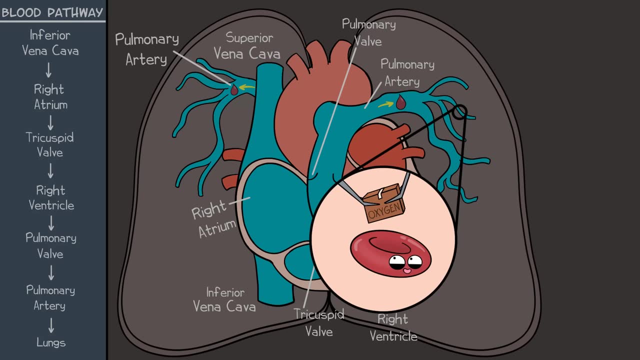 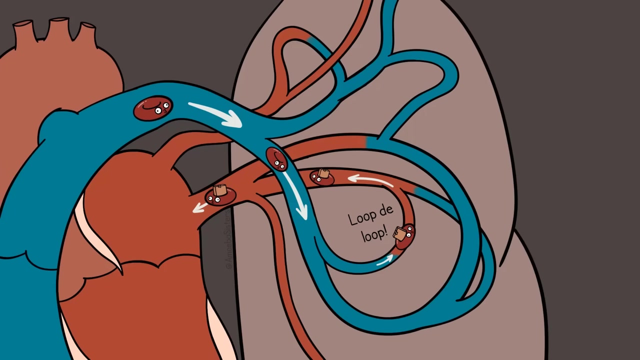 pulmonary. it likely involves lungs. the pulmonary artery takes blood to the lungs. the lungs are where red blood cells in the blood will take on oxygen and release carbon dioxide. now this blood is oxygenated, it needs to return to the heart so that the heart can pump it throughout the body. the oxygenated 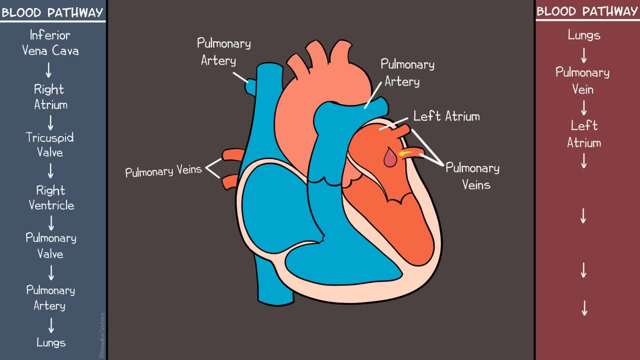 blood travels through a pulmonary vein to the left atrium. the left atrium contracts and the blood travels through the mitral valve, also known as the bicuspid valve, into the left ventricle. the left ventricle contracts and pumps the blood through the aortic valve into the left ventricle and then the left ventricle. 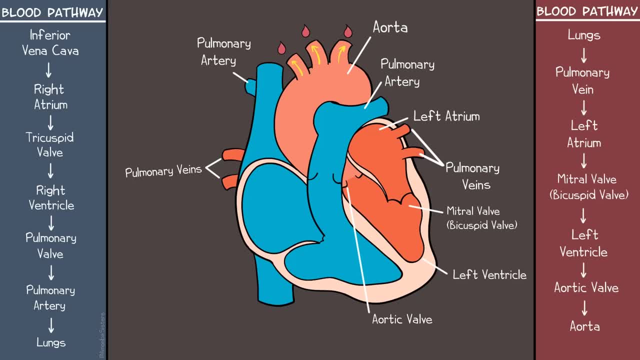 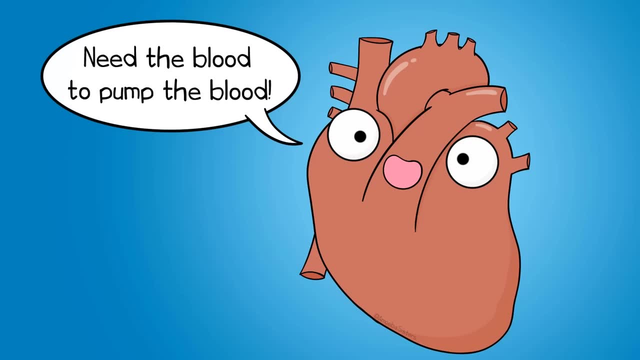 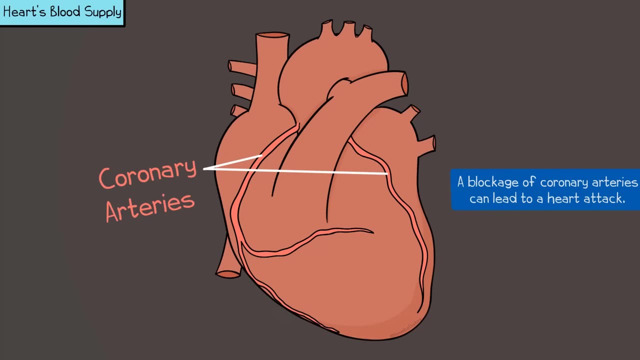 out a major artery known as the aorta. the aorta is a major artery that carries oxygenated blood throughout the body. now I don't want to neglect the fact that the heart needs its own blood supply for delivery of oxygen and glucose. the heart can receive this blood supply through coronary arteries. coronary arteries. 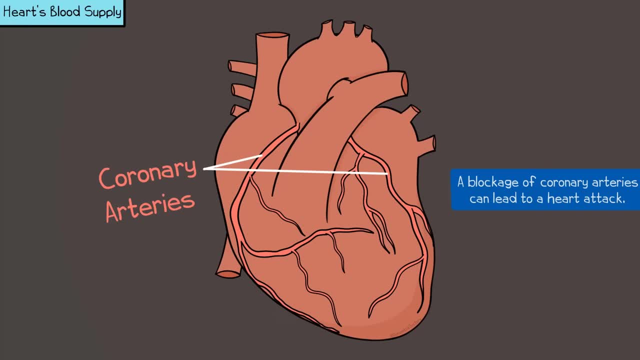 branch off the aorta and eventually deliver blood into capillaries. these capillaries deliver oxygen and glucose to the heart. coronary veins will take the deoxygenated blood to the right atrium, where the blood will eventually travel the pathway to become oxygenated.